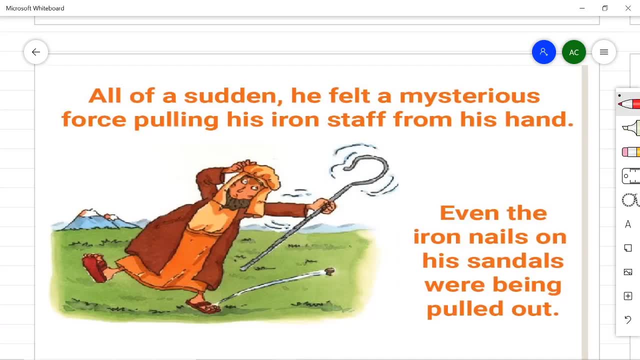 known as staff, and all of a sudden, something mysterious happened and his shoe nails- okay, shoe nails which were there in his shoes, and his iron hook, which was there on his staff or stick- they got attracted towards a piece of rock which is which contained magnetite, and he was very surprised that what it? 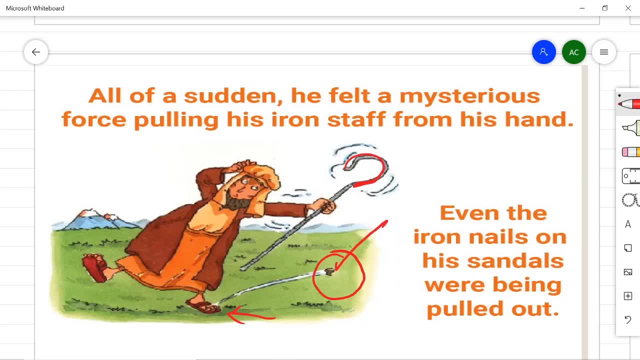 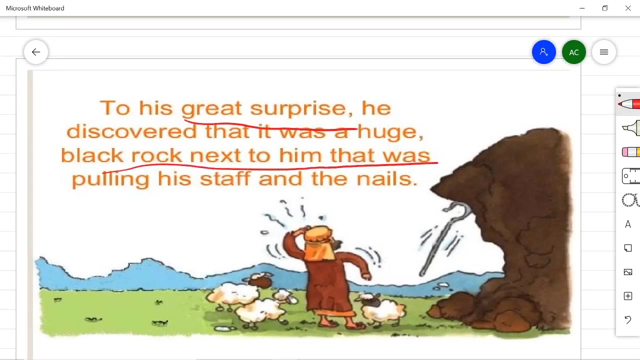 is happened, why it is happening. and why it is happening and why it is happening. later on, this rock was found to be magnetite and this magnetite had the property to attract iron pieces. after that his he was surprised because he discovered that it was huge black rock next to him that was pulling his staff. 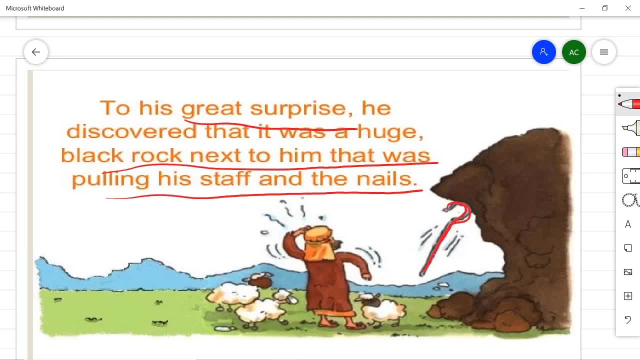 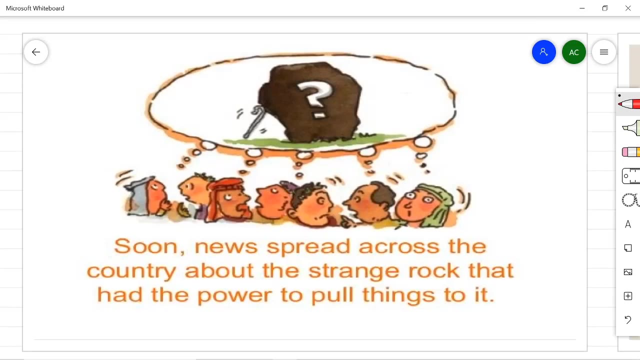 this is staff and nails. so this rock was rock of magnetite and this rock had the property to attract iron pieces or iron substances. now, soon people started talking about this mysterious rock and this is strange rock and they were telling this rock had the power to pull things to it and later on it was told that it was not pulling everything. 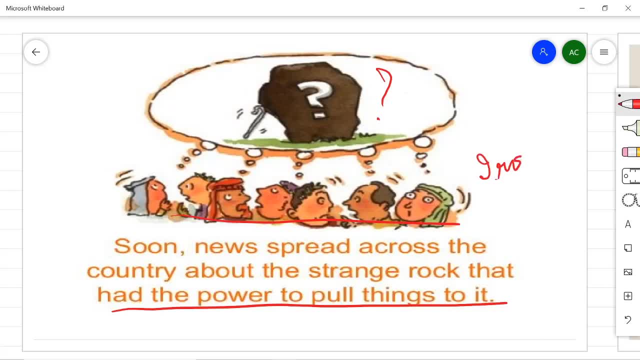 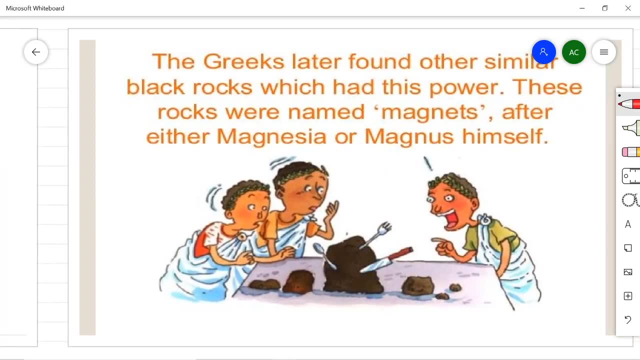 rather, it was pulling only things made up of iron. the area where this, this rock, was found was Asia Minor, and there's a district in Asia Minor known as magnesia, so this was the name of the place where this rock was first found, and the people who lived were Greeks here, because Greece is the 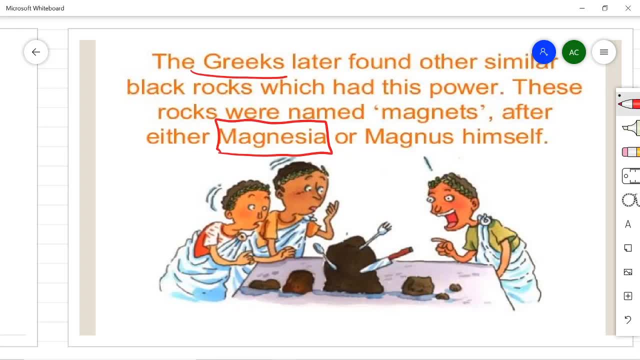 country, major country in Asia Minor. so the Greeks later found that these rocks, these black rocks which had power, were named as magnets. and why they were named as magnet? because they were found in magnesia by Magnus. okay, that's why they are called magnets, that is why it is known as magnet. Later on it was found that lodestone which is known. 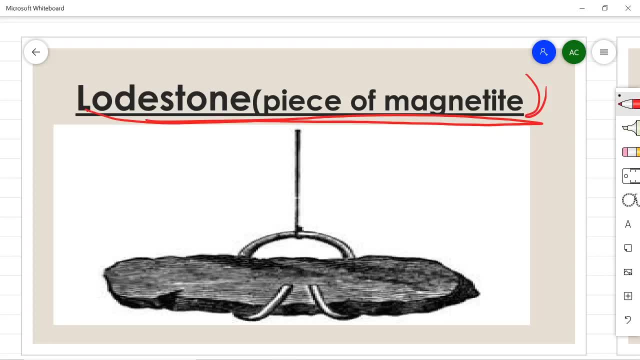 as piece of magnetite and which is natural occurring ore of magnetite or ore of iron. These are this lodestone is known as natural magnet and why it is known as natural magnet? because it is occurring naturally in the earth crust. So they took this piece of lodestone. 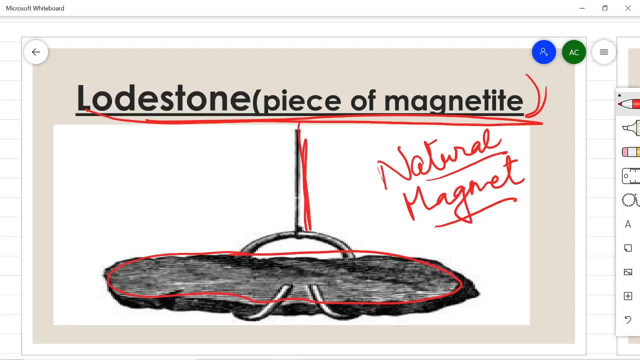 and they then hanged it with the thread. It always rests in the particular direction. So later on this lodestone was used to predict the directions. But because they are naturally occurring magnets, they are weak and irregular shape. It does not have a particular shape. 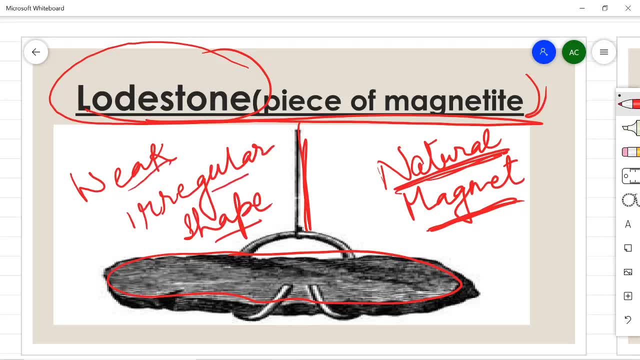 So these were the properties of natural magnet. So natural magnet is a magnet. This is also known as lodestone, and they were found in quite irregular or odd shapes and weak in strength, and that is why not much in use. not much in use because they were. 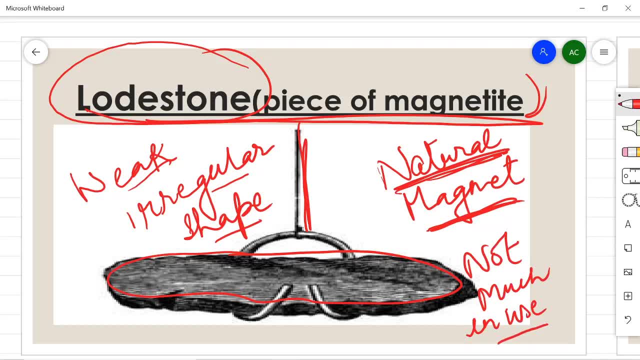 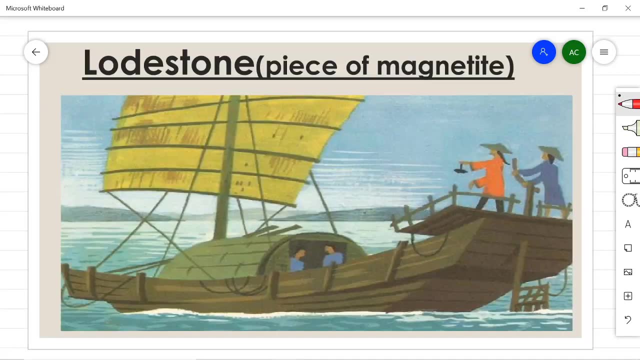 weak and that is why, for practical uses, we started making artificial magnets. and why artificial magnet? Because they were made according to our choice and according to our requirement shape. So this load stone which is piece of magnetite- you can see here this fellow. 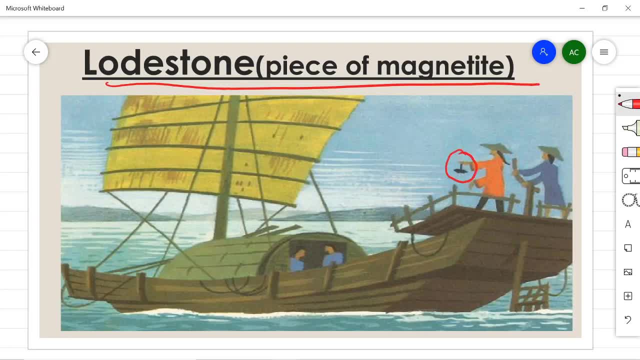 is hanging this load stone for the direction. when on the sea voyages, when they used to go on sea journey and it was difficult to find out the direction, they used to hang this load stone. and when they were hanging this load stone, it always rests in a particular 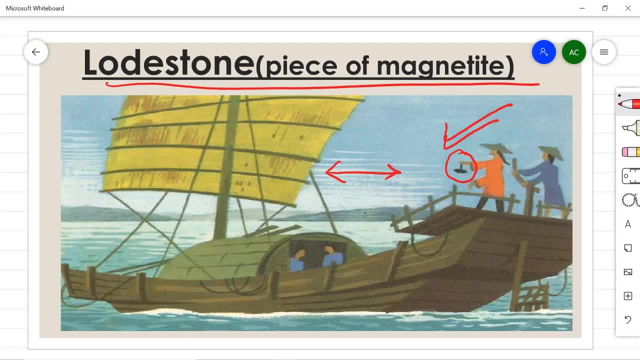 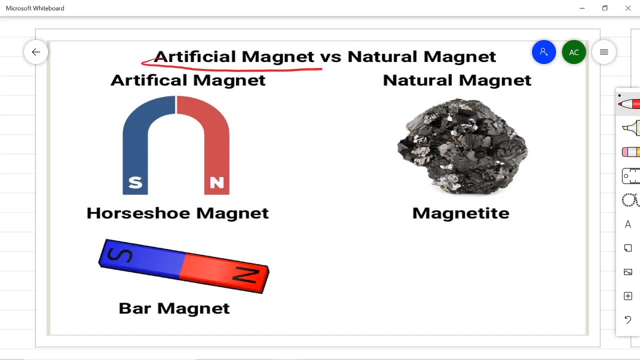 direction and we will study which direction it was actually resting and this way, this load stone was used in predicting the directions by ancient people. So, as I told you already, what are artificial magnets? which are made by man, made by man, and they are known as artificial magnet, and they are made up of? they are made up of iron. 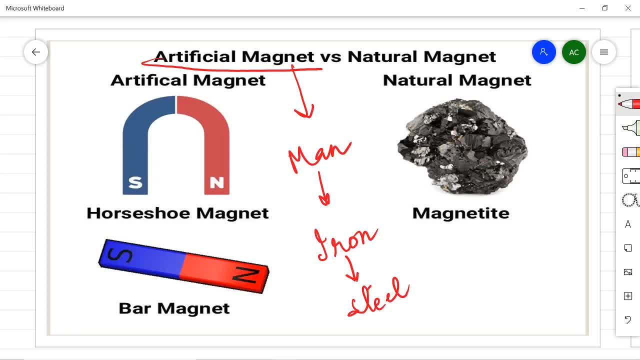 or they are made up of iron. So artificial magnets are made up of iron or steel and of various shapes. you can see here horseshoe magnet, which is in the shape of horseshoe, and bar magnet, which is in the shape of a bar, and they were very, very strong. they were strong and various shapes were there. 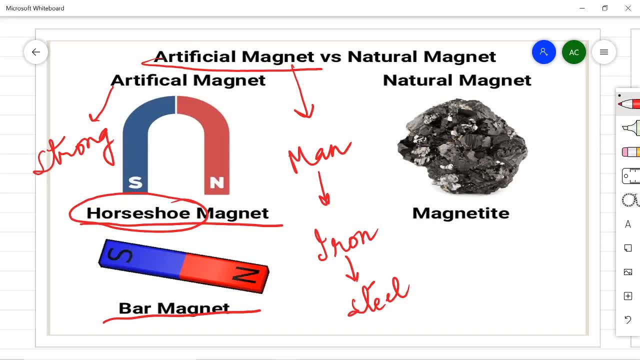 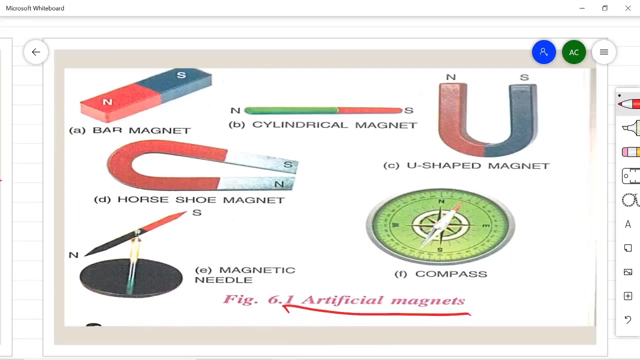 which we will be studying after this slide, And magnetite, which is a natural magnet. you can see irregular shape, weak in strength, so they were not in much use and they occur naturally. nobody makes them. they are made by nature, so nature makes them. So these are the various shapes of artificial magnet which you have to draw in your copy. 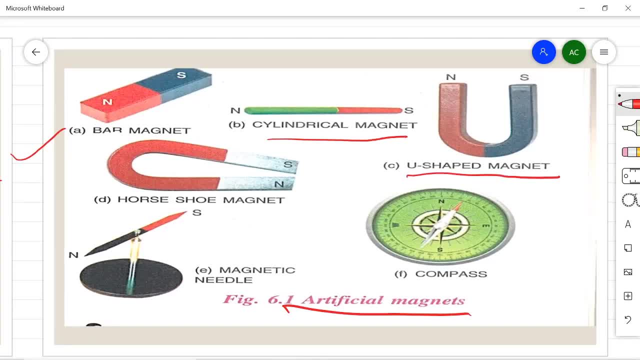 bar magnet, then this is cylindrical magnet, this, this is u shaped magnet, this is horseshoe magnet, This is magnetic needle and this is magnetic compass. so magnetic compass are used to find the geographic directions at a place, because it will, the needle will always rest in a certain 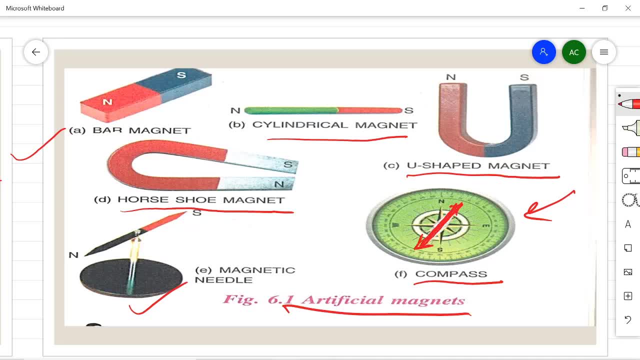 position. so that is why, in a north, south direction, we say so, this magnetic needle. always, whenever you keep this magnetic needle, magnetic compass, somewhere, this magnetic compass will show you the direction, because it always rest in a particular direction. According to that, you can tell which direction is where. 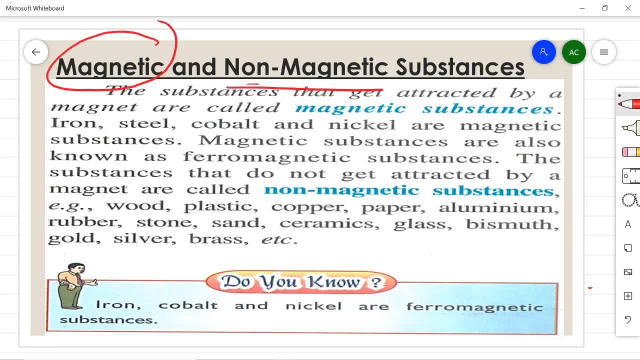 Then let's understand what are magnetic and non-magnetic substances. or which attracts iron pieces, that is magnet. but what are magnetic substance that get attracted by magnets? so those substances which are attracted by magnet, we call them magnetic substances. so which will be the magnetic substances? first of all, you should know it is iron, because iron is. 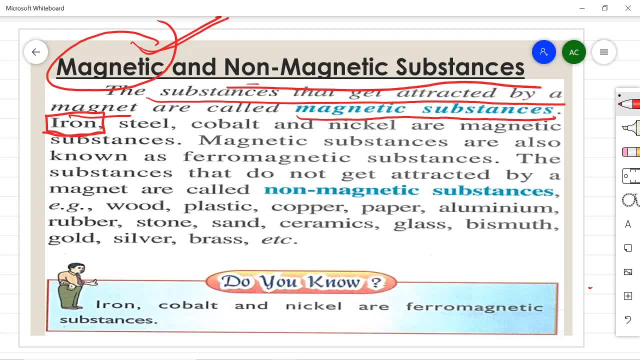 attracted by the magnet. So first magnetic substance is iron, then steel also, cobalt also and nickel also. so till now you were knowing that only iron gets attracted by magnet. but now you should remember that iron, steel, cobalt and nickel are magnetic substances, because they get attracted towards. 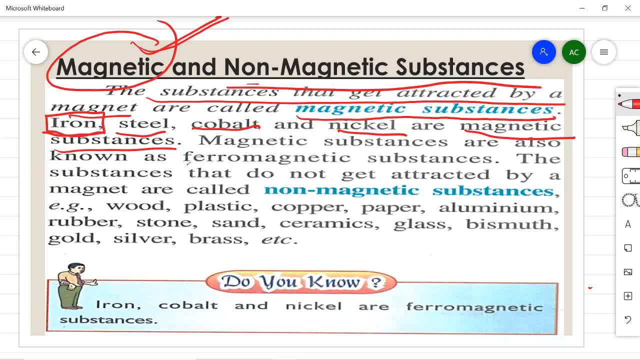 magnet, then they are also known as ferro magnetic substances. that means magnetic substances are also known as ferro magnetic substance, oke magnetic substances. so you should remember the spelling and you should remember the name. what are ferromagnetic substances which get attracted by? 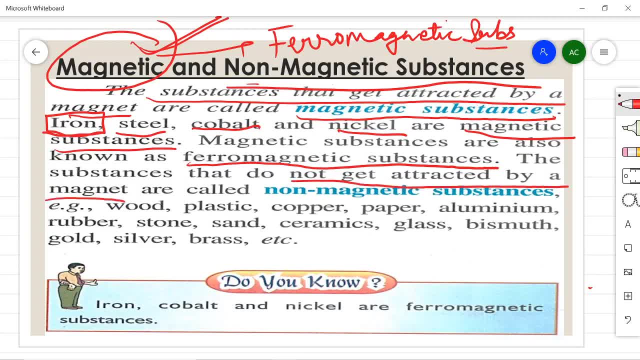 the substance that do not get attracted by the magnet are called non-magnetic substances: plastic, copper, paper, aluminium, rubber, stone, sand, ceramics, glass, bismuth, gold, silver, brass- bismuth is also a substance, okay, so they all do not get attracted by the magnet, and that is why. 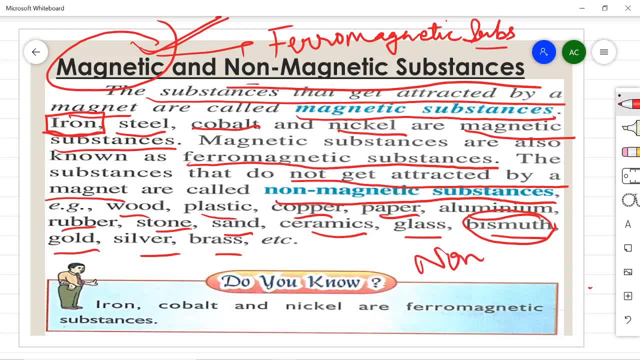 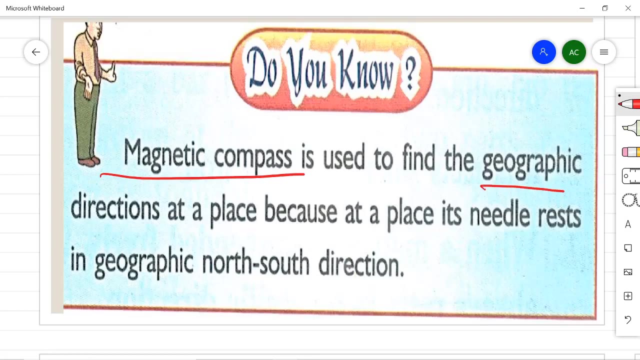 they are known as non-magnetic substances. so this examples and definition you should remember. now, these are the examples of ferromagnetic substances, that is, iron, cobalt, nickel are the ferromagnetic substances because they get attracted by the magnet, as i have told you, magnetic compass. it is used to find the geographic directions as a place, because 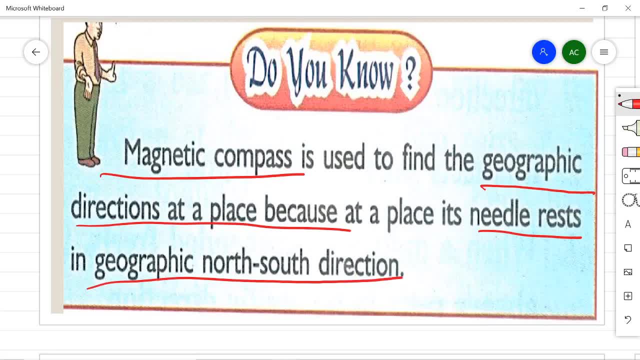 the needle rests in geographic north, south direction. suppose this is north, this is south, this is west, this is east. so whenever you have a compass, its needle will always rest in this direction. that will be towards uh, north and your magnetic south, that will be towards south pole of the earth. so this way, magnetic needle will always rest. 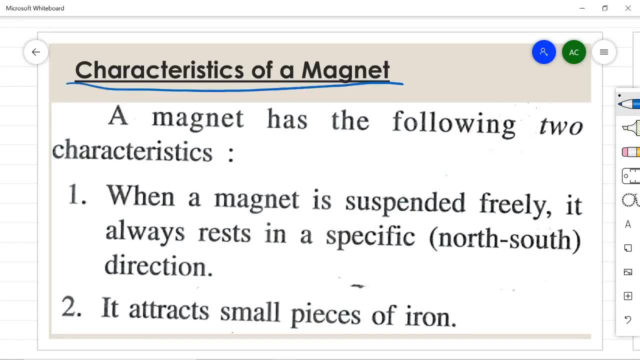 then characteristic of a magnet. what are the characteristics of a magnet? how you will come to know that this substance is magnet. so, first characteristic: it is its uh direction telling capacity. uh magnet, whenever is suspended freely, then it will always rest in a specific, that is not south direction, which i have told you. 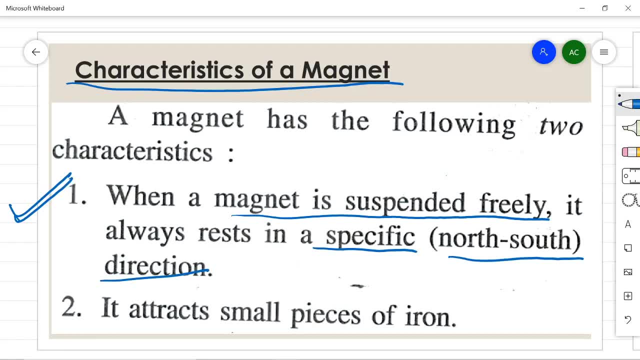 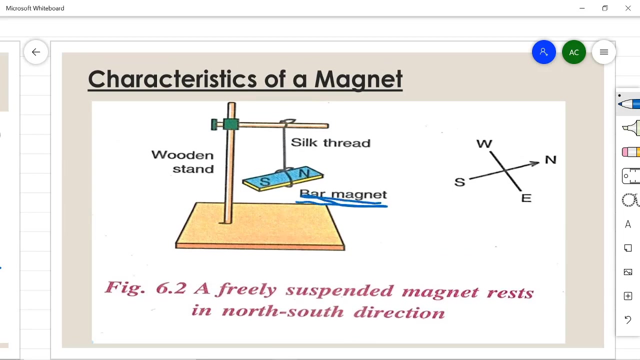 right now, in the last line, that the needle will always show north, south, direction. the compass needle which is north will show the geometric north and which is a compass needle south will show geographic south. second is, as you all know, this is very important property magnet activity. so we have taken a bar magnet, we have, uh, we have tied a silk thread and we have hanged it. 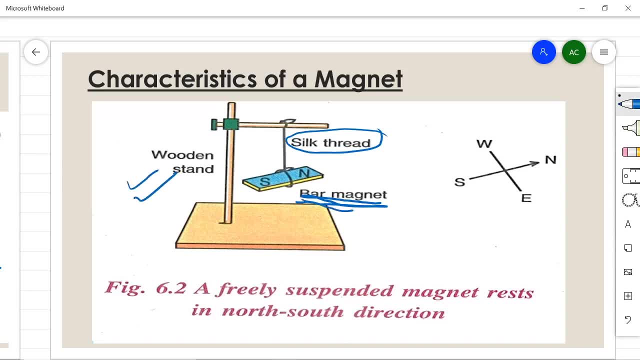 on a wooden stand or square up around free channel channel 일�piece channel. il will stop till the end. help, so our magnet are'll veith n is resting. Why is it resting in this direction? Because where you have set up this is the. 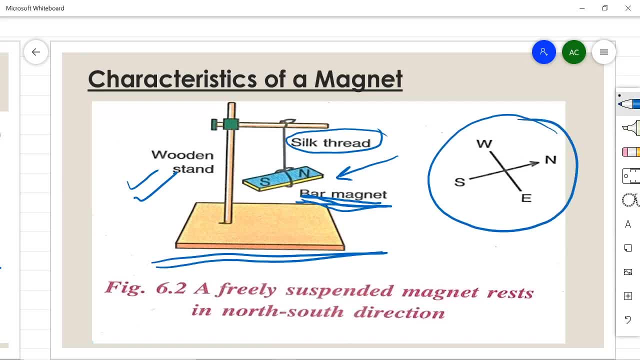 position of that room, or you can say the place On this side is the North. Geographic North and Geographic South is like this. So the bar magnet will always point towards the North. So they will be in the same direction: North and North Pole of the bar magnet. So freely. 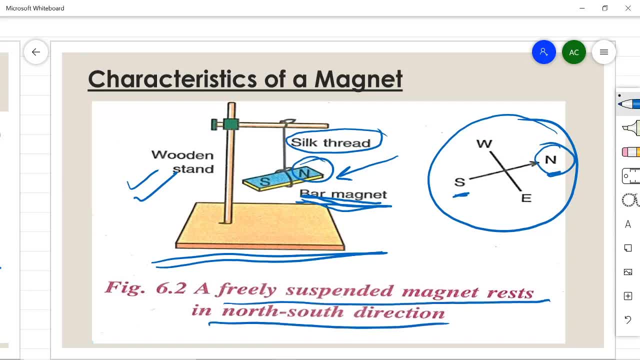 suspended magnet always rest in a North-South direction. So this activity will tell you that magnet will always rest in a particular direction. and what is that direction? North-South direction. Now, you have disturbed it, you have moved it. it will rotate in a while it. 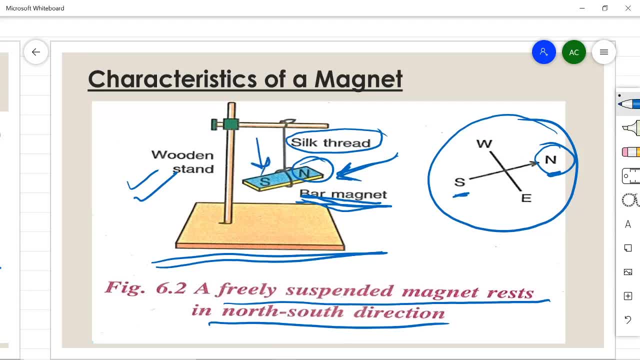 will move and after that then also it will come back in this position, In the same position again. it will come back because it always rest in a North-South direction. The end of the magnet will always be in a North-South direction. So this activity will tell you. 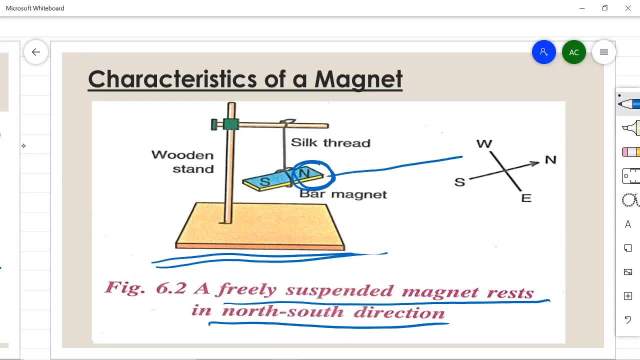 this is the point of magnet which points towards the North, point towards the North. we will call it the North-seeking Pole or the North Pole of the magnet. There are two names we will remember. North-seeking Pole: Seeking means seeing or searching. North-seeking. 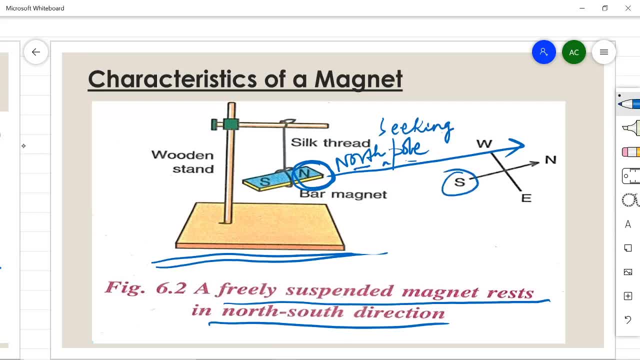 Pole, or simply North Pole, and which is going towards South. It will be yours South-seeking Pole, or simply South Pole pole. And how do we show it on the magnet? It is written in the form of N and S. If you look at the bar magnet, there are dots in it and it says north and south poles Sometimes. 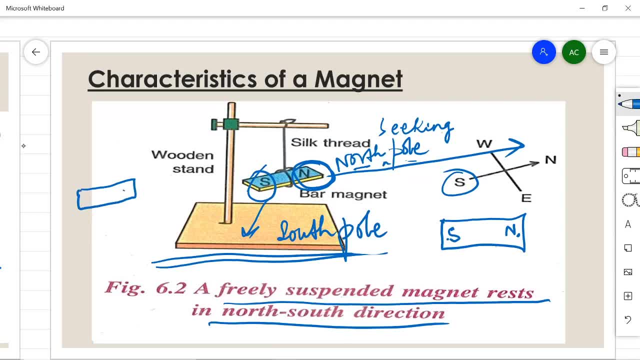 the magnet has a red dot and the red dot shows the north pole. So sometimes in a magnet it is not written it is north pole, but a red dot is marked to tell north direction And naturally if it is north then its opposite will be south. here Then the next characteristic. 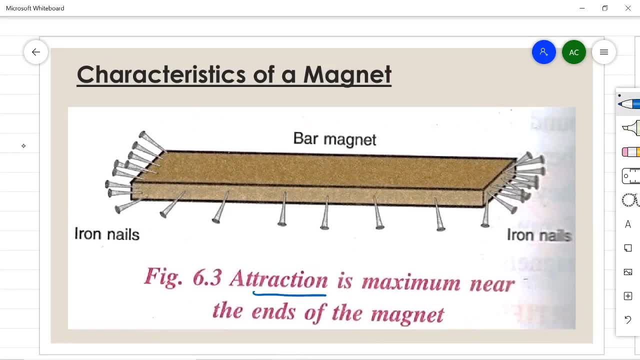 of magnet is attraction of iron. So we will take the magnet once like this and we will attract iron nails from all sides, So at all places. you will see that here on the poles, like this is the north pole and this is the south pole, This is north pole, south pole. 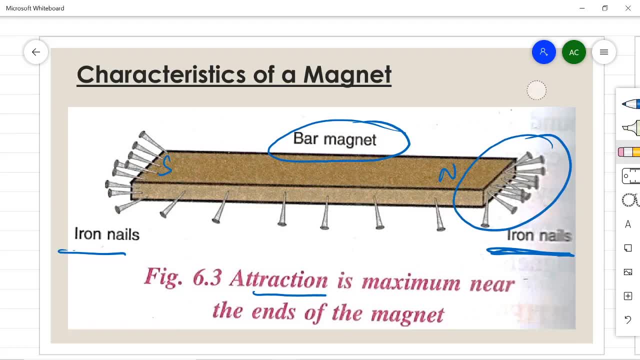 So you will see, the maximum number of iron nails are attracted on the poles, And in the middle there are less nails. So this means that attraction is maximum near the ends of the magnet. And why is it so? Because the magnetic properties are maximum on the poles. 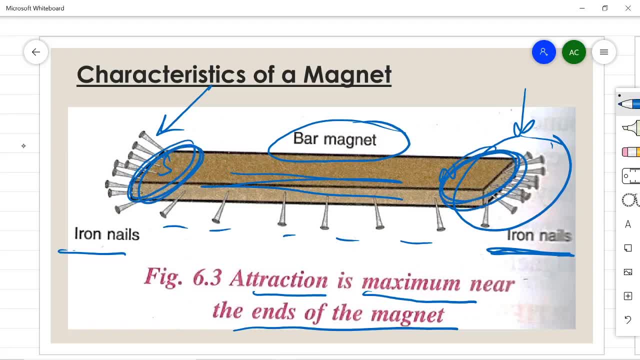 Here, on the poles, the power of the magnet is the strongest, So that is why the magnet is the strongest, and in the middle area the power is less as compared to the poles. So this is the and in this way, the poles are both the ends where iron is attracted and 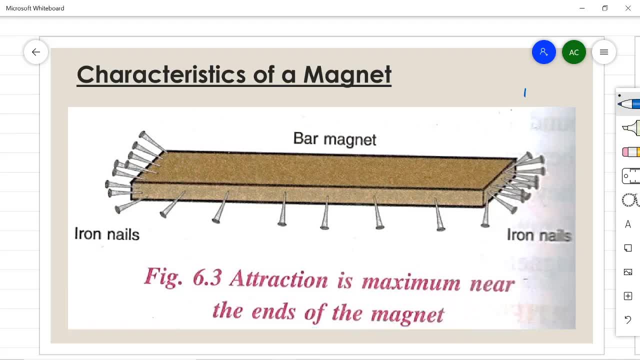 the power is maximum. These ends are known as magnetic poles. Okay, So what are magnetic poles? Magnetic poles are the places where this is also a magnetic pole and this is also a magnetic pole. This is also magnetic pole. So the ends of the magnet, where the attraction property 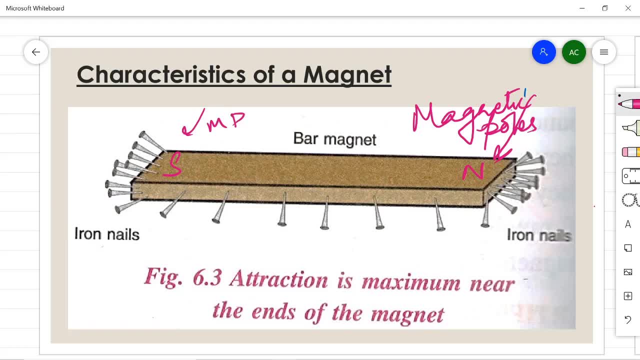 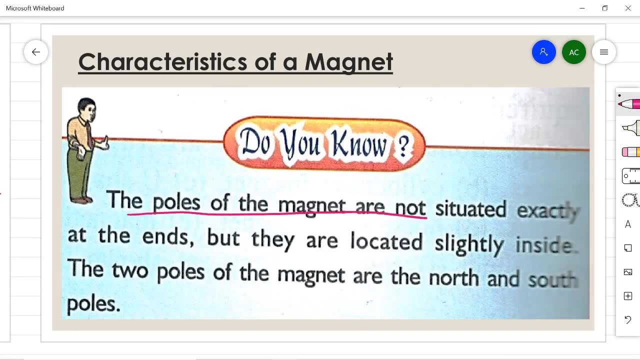 is maximum are called magnetic poles of a magnet. Now there is a very interesting story about these poles. The poles of the magnet are not situated exactly at the ends, but they are located slightly in the middle of the magnet. So the magnetic poles are the places. 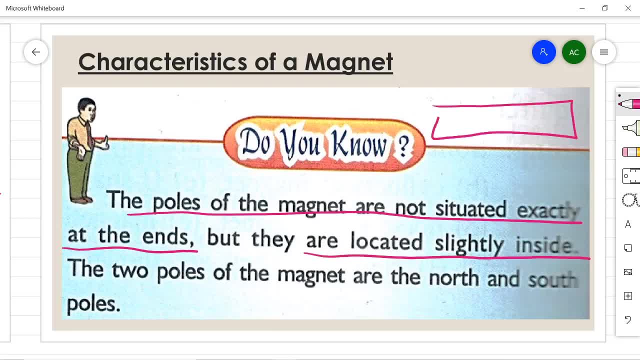 on which Inside come. the Polish hadn't occupied from the beginning. If there is some member or a magnet of the magnet, its attraction element is located slightly inside the magnetic pole. it is located Montgomery. If you have hook or hoop of magnet then you can check those again. so they are new places of magnetic poles in Europe. so 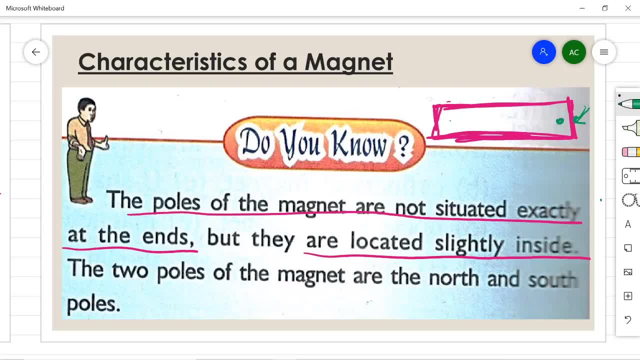 these are near the ends of the magnet So these can be connected electronically in the magnetic pole. they are next to each other, So it will not be happening here, Not here, but here, only inside the magnet. Hey, Thank God, he said that the자n in India as one. 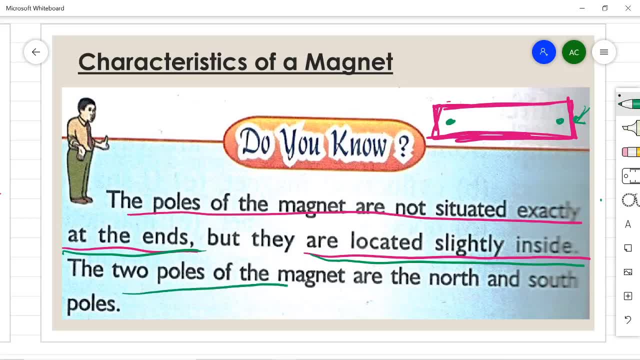 can be hidden from the world. So In this way there are many other magnetic powers within the magnet. so際ly inside One should not be hidden so that one lives here in outermost home within the magnet, than even pointing to another magnet may not get it. So let's. 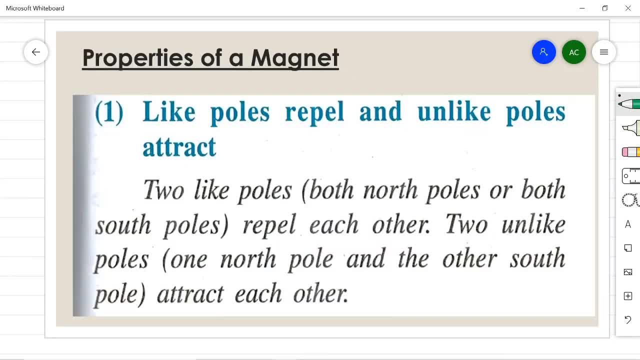 North and South Pole. Now let's understand about the properties of a magnet. First property is: like poles repel and unlike poles attract. If you take two magnets- North Pole and North Pole- and bring them together, so what will happen? There will be a repulsion, It won't be an attraction. 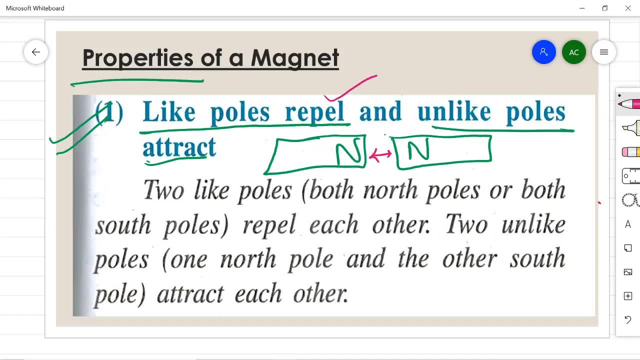 it will be a repulsion. Repulsion means they will go far away and repel each other and push each other in the opposite direction. But if you do the opposite- you have one North Pole and the other you have kept South Pole here- then there will be attraction. They 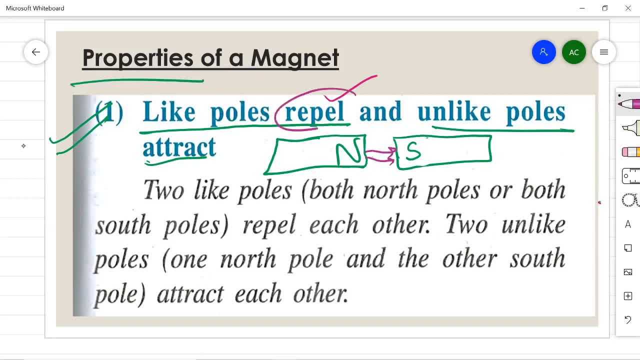 will get attracted. So always remember: like poles repel, unlike poles attract, So North, North or South, South, they will repel each other. south, south will repel each other and north will repel, But when it is north, south, they will attract each other. Let's see one activity where we will be showing this property of 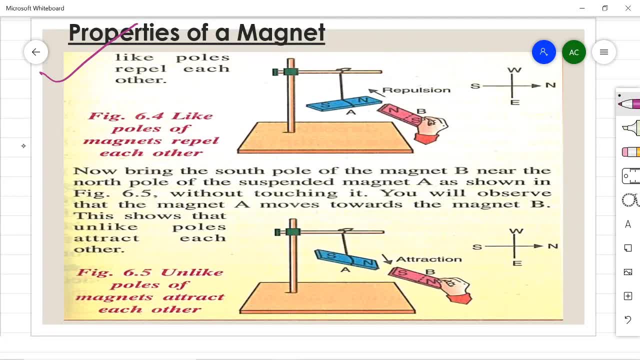 like Poles repel each other. We will take a set up like this and we will bring the magnet. We will hang one magnet and towards its north we will bring one magnet and that magnet's North Pole will be attracted to the opposite direction. We will apply the magnetic pulse. 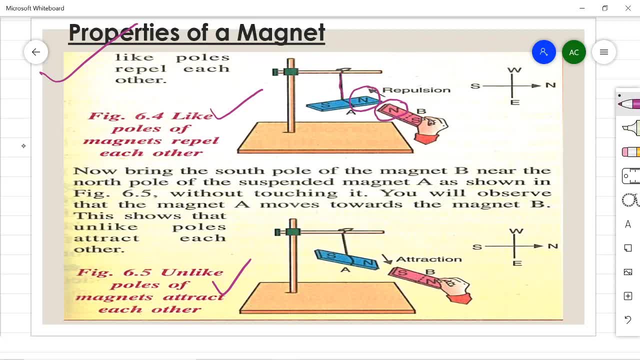 If you like to do this, then you are awkward and you are going to get the magnet. their magnet will respond when he turns in to you. He will respond when i shake out his hand for near this North Pole of suspended magnet. You will see that this magnet will go. 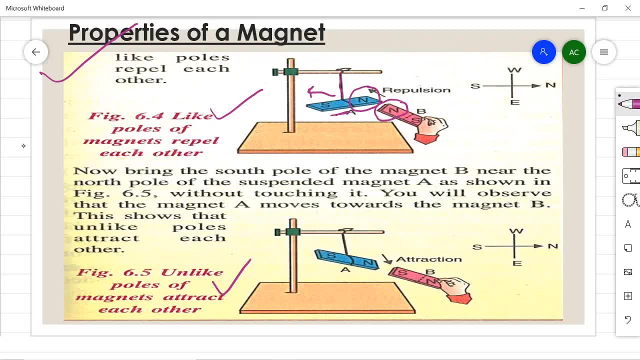 little behind. Why? Because it is repelled. Keep it a little away, don't touch it. Do the same here. Don't touch it, keep it away, But you will see that the suspended magnet has come near it. Why? Because there are opposite poles, North and South. So this 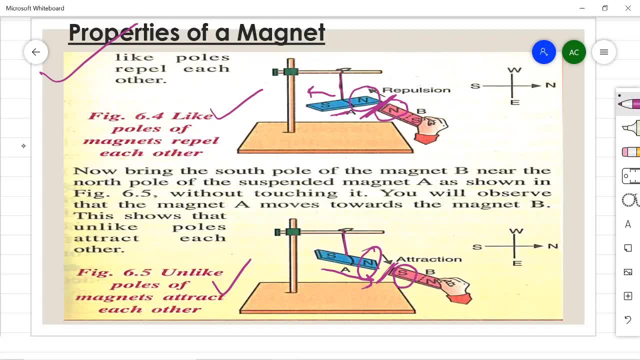 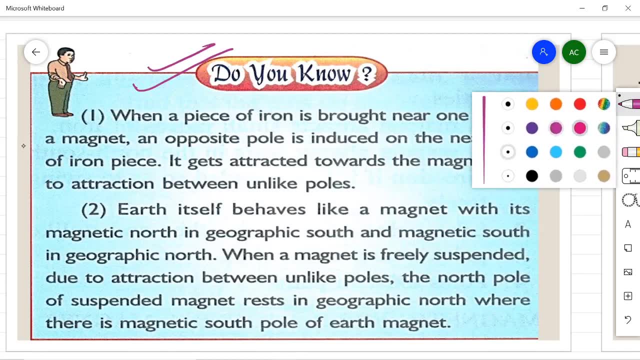 will show that, unlike poles attract and like poles, repel each other. Now this, this is very important concept which you have to understand here. that suppose you are bringing this one is a bar magnet and this is its North. Now you are bringing a piece of iron here and 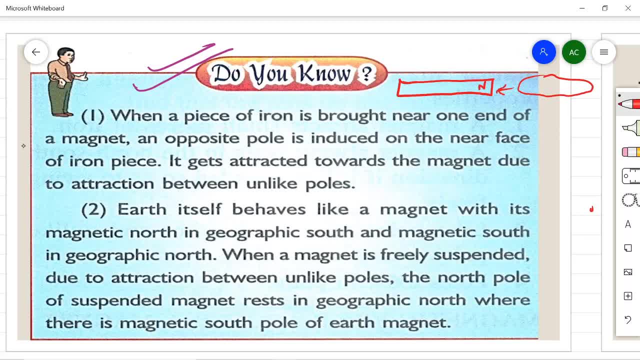 this piece is attracted, Why it attract, Why it is attracted. Always remember this iron piece. As soon as you bring it near a magnet towards any pole, whether towards North Pole or towards South Pole, a temporary pole develops here which is opposite. If it is North here, then 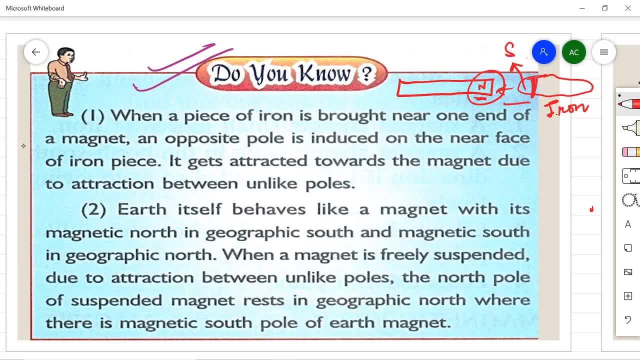 this pole will develop South on the iron and it will attract. Similarly, if you have taken a South Pole of a magnet and brought an iron piece, then this iron, the pole that will be created here, will be a North Pole and that is why it will. 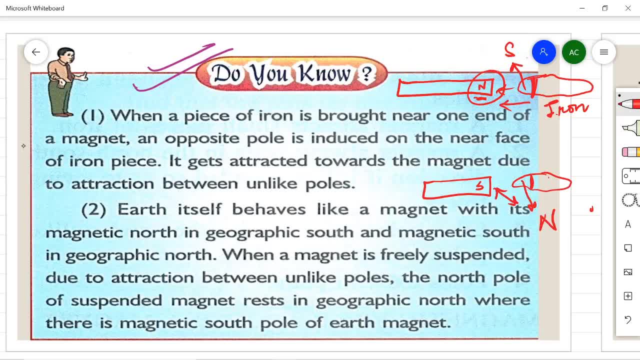 attract because it will become opposite. Okay, But these are temporary poles which will take away the iron and the pole will get destroyed. So this way you have to understand that when a piece of iron is brought near one end of the magnet, opposite pole is induced. 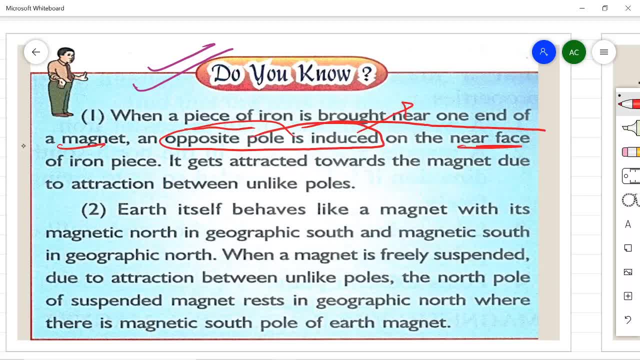 Induced means created on the near face of iron piece, Whatever face you are bringing near the magnet, and then it gets attracted towards the magnet due to attraction between unlike poles. Then, second point, which is very important, earth also behaves like a magnet. earth is: 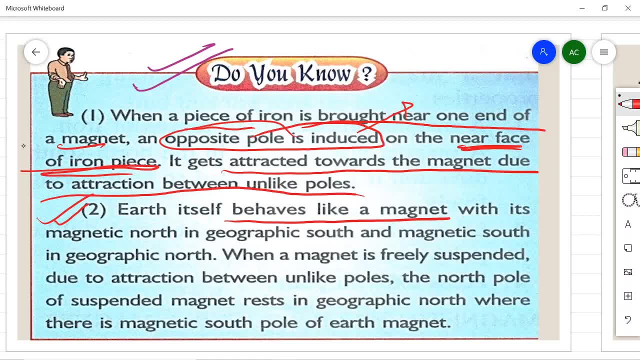 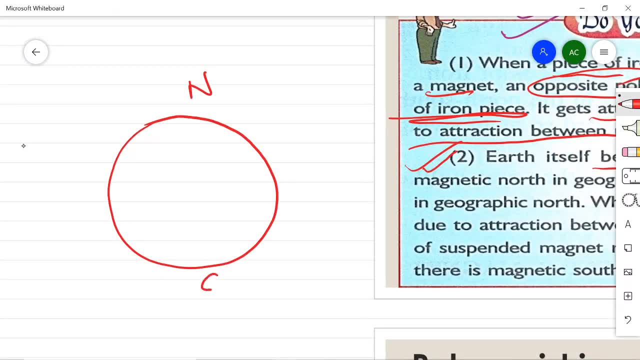 a very big magnet. but you have to understand this in earth, that the magnetic of earth, suppose this is earth, this is north, this is south, which you have studied in geography, north and south, but the earth is a magnet if we now this is earth, this earth its. 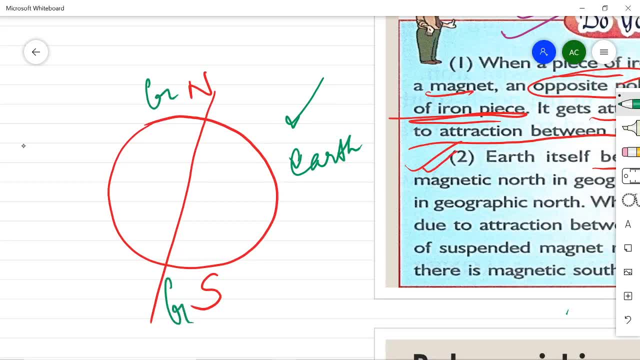 poles- this is south pole and this is north pole- means opposite south pole and north pole. This blue which I am writing, this is magnetic north and magnetic south. so Gn for geographic north and magnetic south is magnetic north and magnetic south is magnetic south. 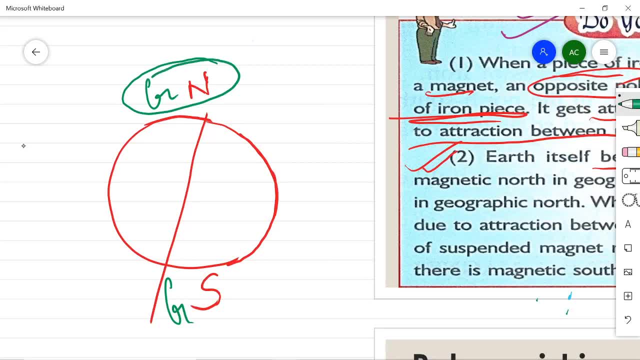 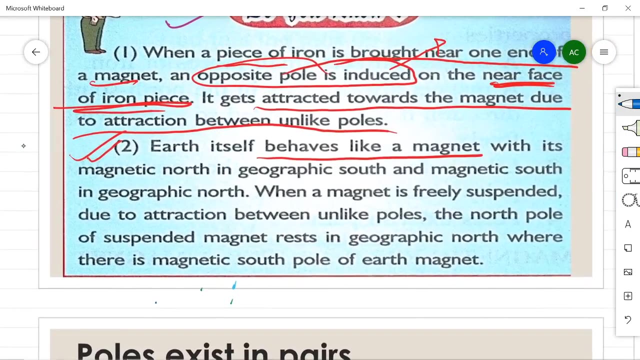 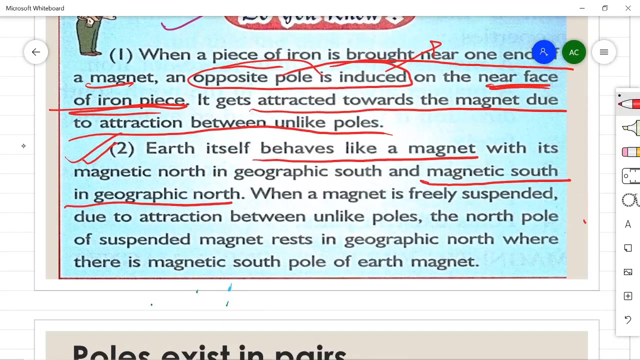 Okay, Okay, Okay. So earth behaves like a magnet and magnetic south is in geographic north and geographic south is in magnetic north. Remember opposite. so when a magnet is freely suspended due to attraction between unlike poles, the north pole is suspended. magnet resets in geographic north, where there is. 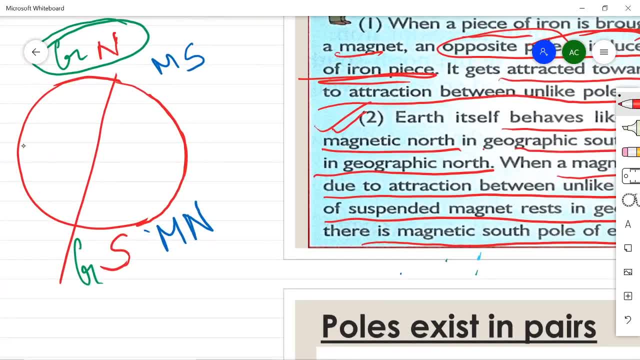 magnetic south pole of the earth magnet. now you will understand what happened. suppose I have introduced a magnet here. okay, this is a magnet. this is the north pole of this magnet. Okay, Okay, Okay, Okay, Okay, Okay. 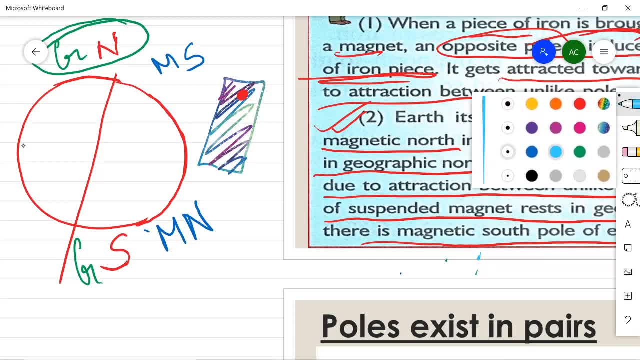 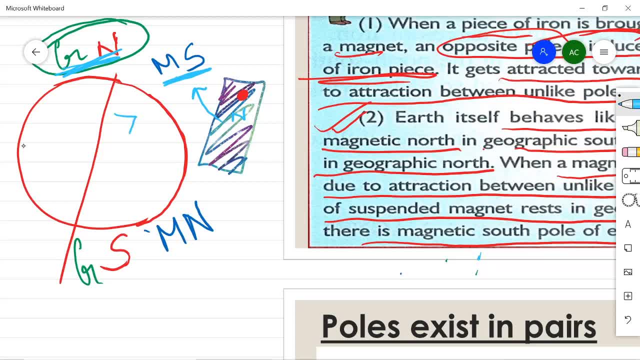 the magnetic south. hence, whenever you hang any bar magnet or any magnet on earth, it always shows towards the north direction. Which north direction Towards the geographic north right? You have the right to know, But actually it is being attracted towards the magnetic south. 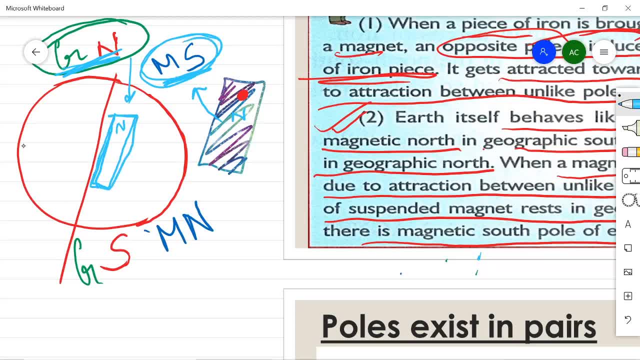 That's why it always rests in this direction, Because that doesn't mean that it is from the geographic north. It means that the earth is a magnet And it knows that in the geographic north there is a south pole, So it is being attracted from the north to the south. 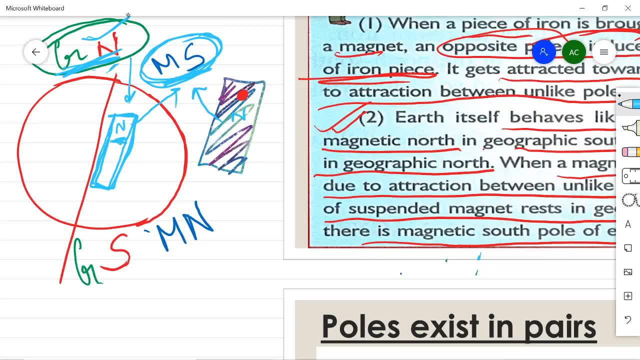 That's why the north of the bar magnet always points on the geographic north, And this is the opposite. This is the south, This is being attracted towards the magnetic north. That's why it will always hang on the north-south direction. But actually the earth is a magnet. 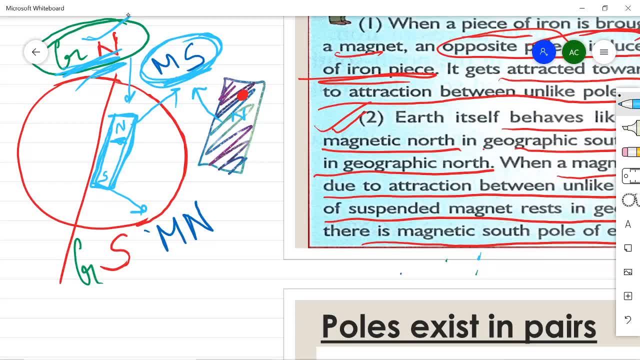 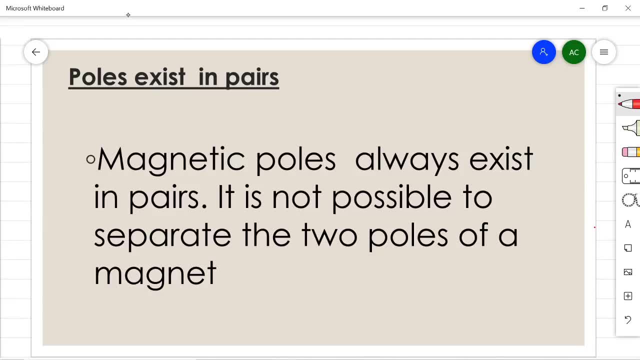 And its poles are opposite. So because it is opposite, it gets attracted. That is why the bar magnet always rests in the north-south direction. Now the next topic is that poles always exist in pairs. It is not like you took a bar magnet. 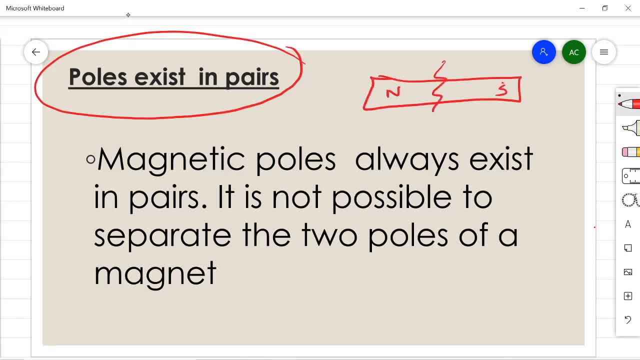 This is the north and this is the south. Now you broke it in between And you said that you separated the north pole and the south pole. No, it is not possible. In the two pieces that you have made, the poles will develop again. 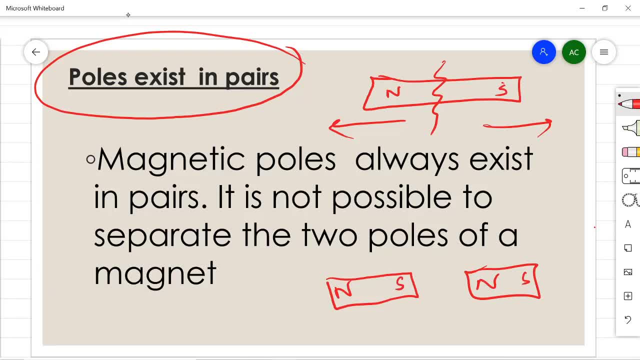 The poles will develop in this way. So poles always exist in pairs And it is not possible to separate the two poles of a magnet. You can never separate. You will always have smaller magnets, but with two poles. So let's see the activity here which we can do to understand. 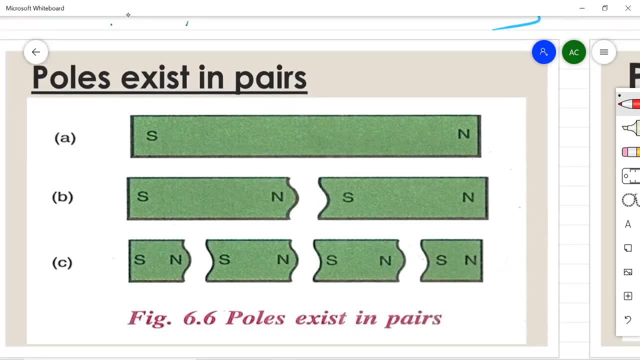 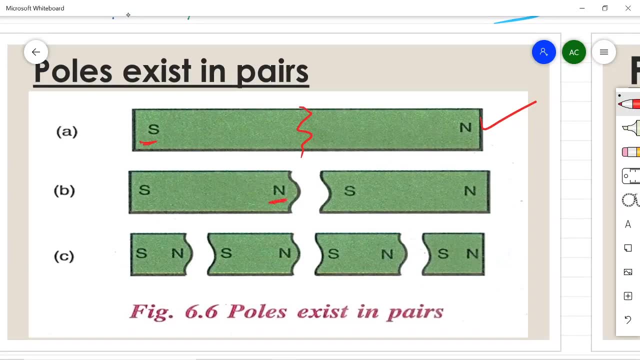 We will take one big bar magnet like this, And now we have broken it from between, So this is south, But here the broken piece will have north. now This is north, So broken piece will have now south. Again, I broke this from here. 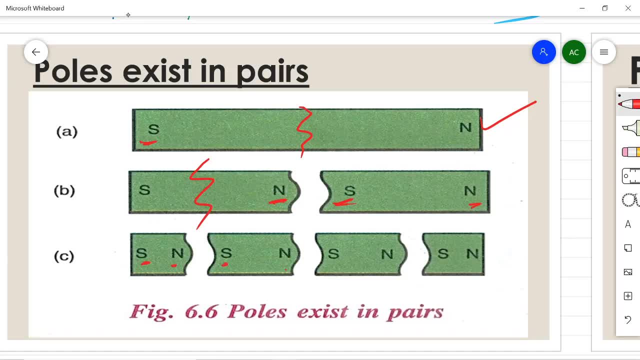 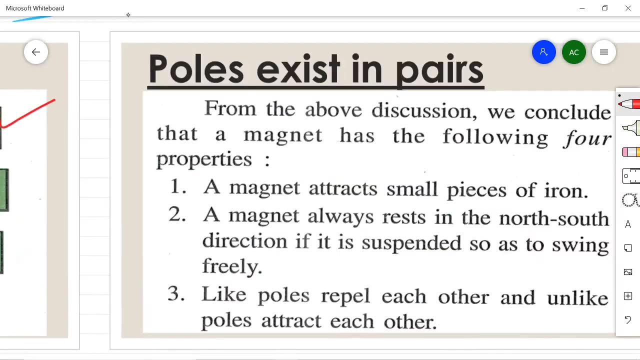 So this again: poles were developed. So you can see Now I broke it from here. So then again this piece will be developed. So that means poles cannot be separated from each other. Every magnet will have two poles. So from the above discussion, properties of magnet are: 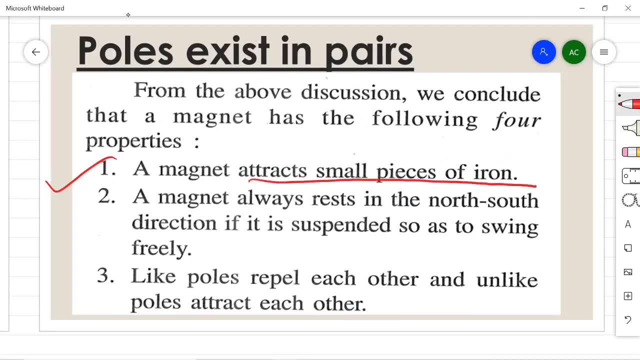 A magnet attracts a small piece of iron. A magnet always rests in north-south direction When, When it is suspended to swing freely And like poles repel and unlike poles attract each other. And this property, that is, poles, exist in pair. 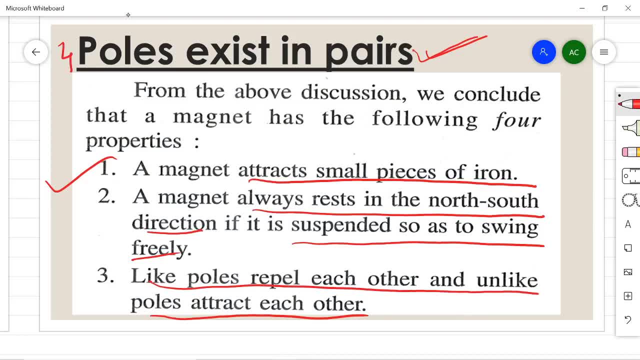 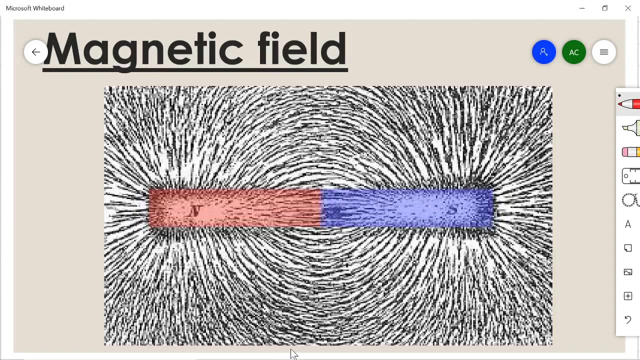 This is the fourth property. This is the fourth property that poles exist in pairs. So always remember these are the properties of magnet. They are very important, So you should learn them. Then the next topic is magnetic field. So what do you understand by magnetic field? 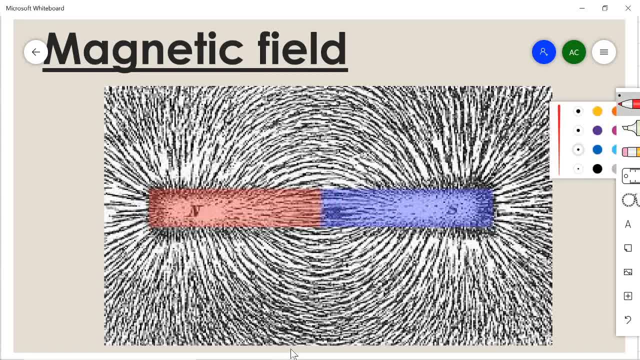 The space around the magnet, as you can see here. This is space, This is magnet, This is magnet. This is north pole of the magnet, This is south pole of the magnet. Now, the particular area near the magnet, This whole area. 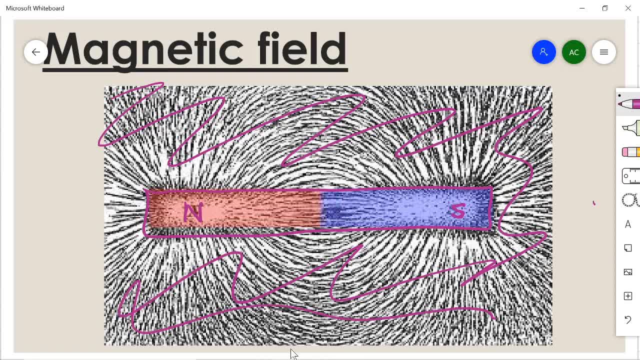 This area is near the magnet. This is such an area that whenever you touch iron in any area, You don't have to touch it with magnet. If you are bringing iron in this area, Then also it gets attracted. So the space around the magnet in which a magnetic substances 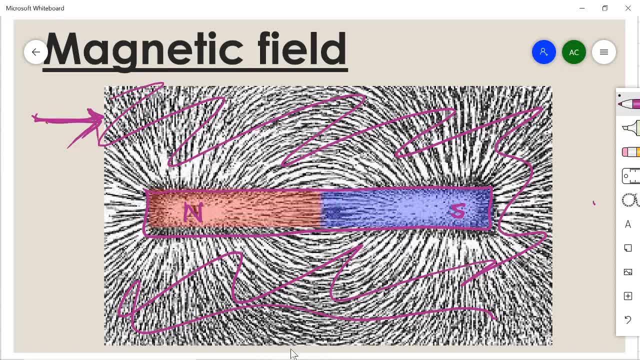 Such as iron or pieces of iron are placed And they get attracted towards the magnet Is known as magnetic field. How will you prove this? You put this magnet on a paper And put small, very fine iron fillings And tap it.